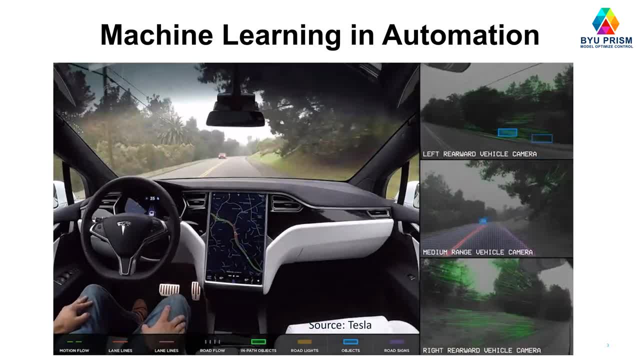 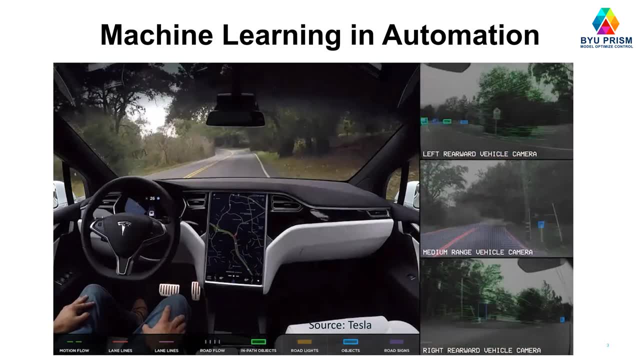 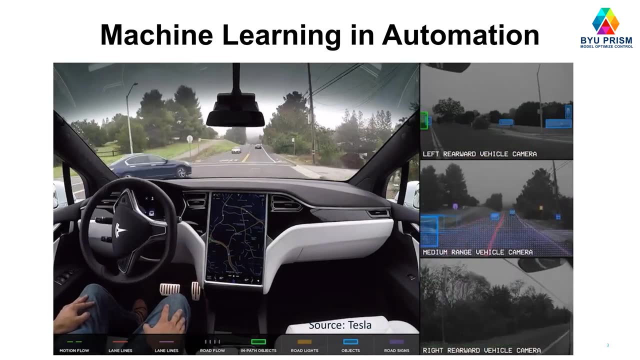 video You can see the driver is navigating without touching the steering wheel, gas pedal or brake. You can see that the automated functions are possible because of machine learning that you can see on the right. with image detection and classification, It's able to identify stop signs. 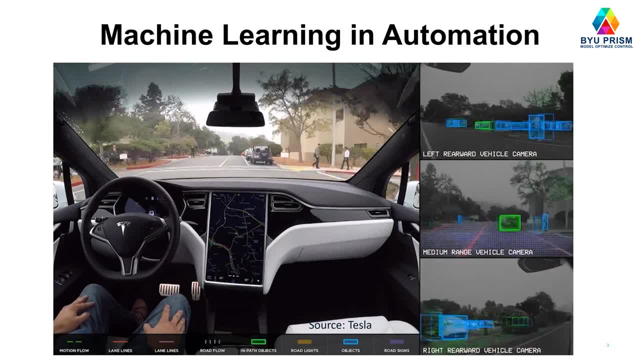 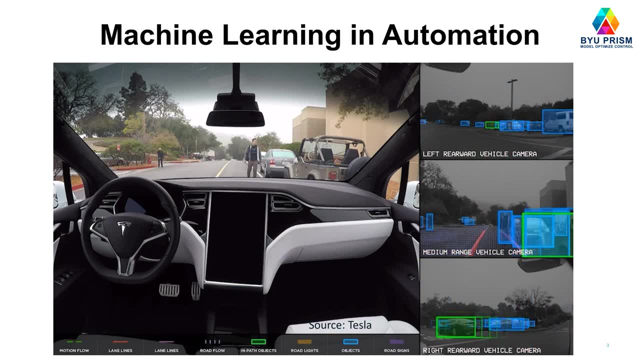 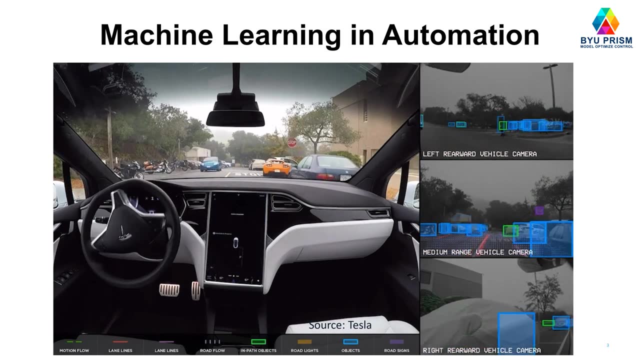 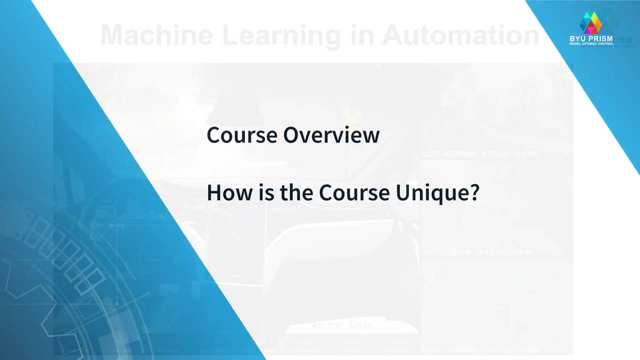 It's able to identify the lanes and also other objects of interest like vehicles or pedestrians. At a certain point, the driver leaves the vehicle and the car goes to find a parking spot, Identifies a parking spot and then is able to park until the driver leaves the building again and summons the vehicle. 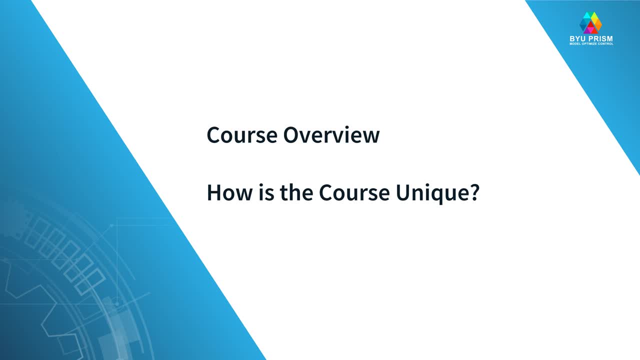 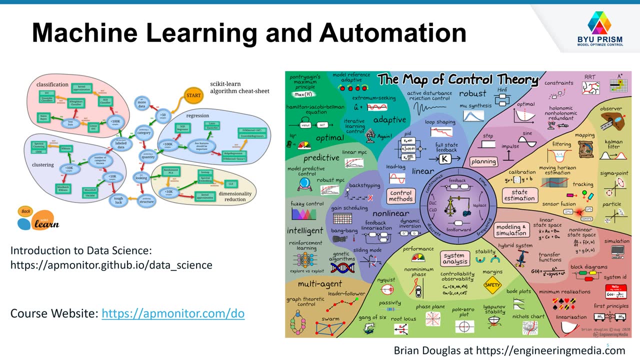 So in this course we're going to talk first of all about an overview, but also mention some things about how this course is unique. So, as we look at machine learning and automation, we look at the field of machine learning, which is rapidly growing and very popular, and you might need some help navigating this. 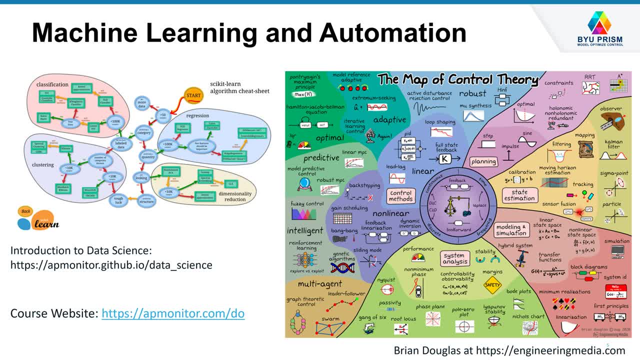 So we're going to start and maybe, if we're predicting a category, we'd say, yes, okay, do we have labeled data? yes, then we would do something like classification. But let's say we don't have a category. it's a continuous value that we're trying to predict. 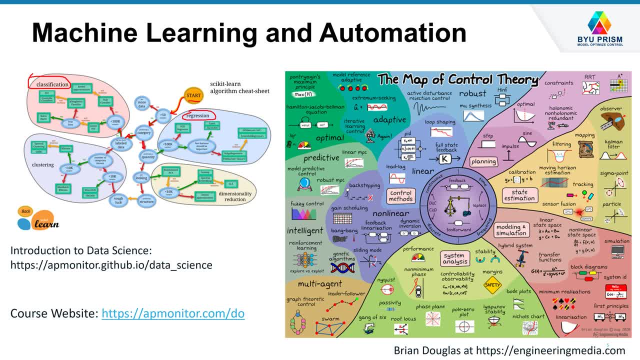 and then we might use something like regression to develop that model. We also have clustering or unsupervised learning methods and dimensionality reduction as well, Okay, So if you just like an introduction to machine learning and data science, there's a good short course here. 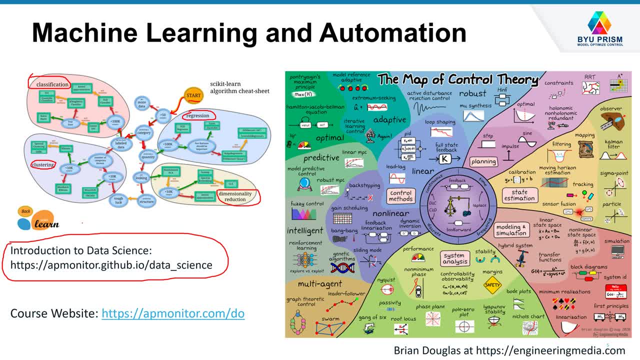 It'll take you a few hours to run through all of the Jupyter notebooks and Python examples. This course, however, focuses on the intersection between these two, So we're going to be developing models that are going to be used in model predictive control. 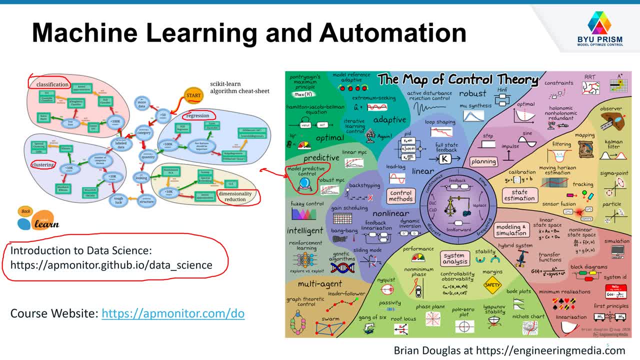 This is a nice map of control theory that's provided by Brian Douglas, and let me just show you some of the areas that we're going to be covering in the course. We're really going to start with modeling and simulation- How to develop a model of our system. we're going to be using discrete and continuous 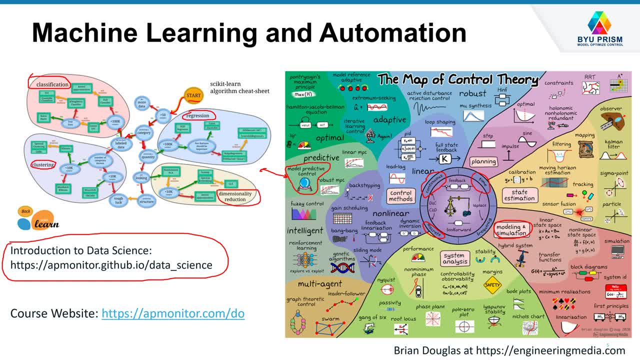 and almost all of it's going to be in the time domain. So with that we'll develop things like linear state-space models and develop models from first principles or physics-based models. but we'll also develop regression approaches And machine learn methods to develop some of these models as well that we'll use in the 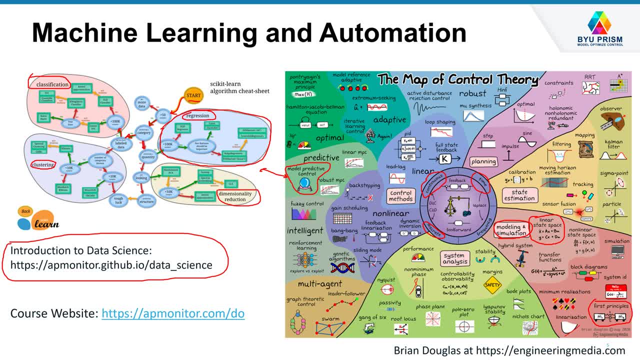 model predictive controllers. Now, we're not going to have an exact representation of our system And so with that, we'll use state estimation to help us improve our models as we're going, And we'll use approaches like moving horizon estimation and the Kalman filter. 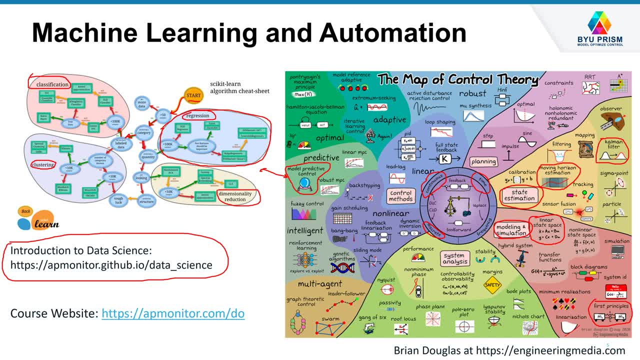 And then going over to control now. Now we're going to take an approach to solve linear and PC, but also model predictive control, And a lot of this has to do with optimization. So there's some optimal control theory and constraints and others that we'll use in developing. 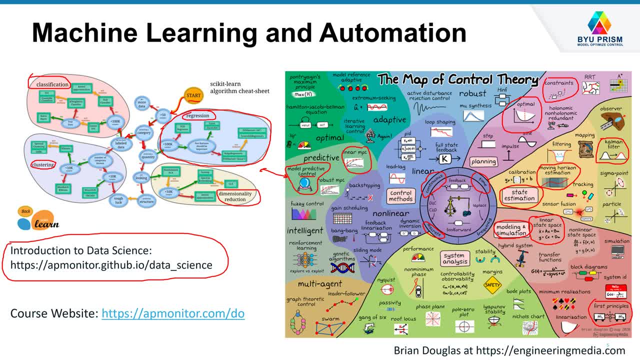 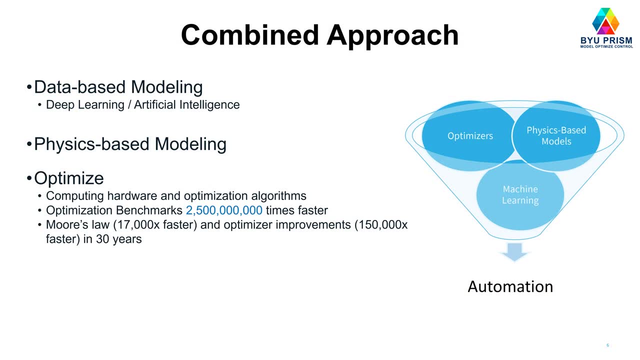 our automation solutions. So if I had to give a map of what we're going to be talking about, it's these things that are circled here, And it's really the intersection between them, which is one of the things that makes this course unique. 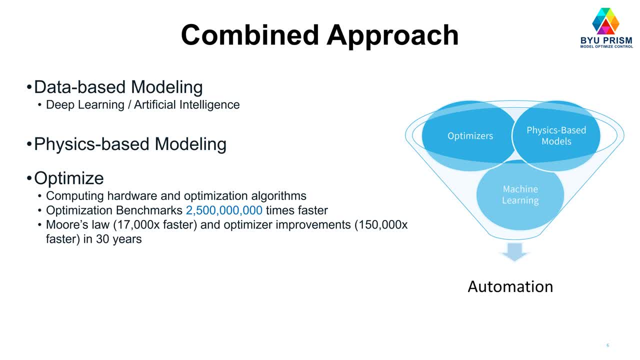 So we're going to be using database modeling, deep learning, artificial intelligence, to develop these solutions. We'll use physics-based modeling as well that develop from material and energy balances and momentum balances. We're going to also use optimization solvers, And one of the perspectives on this is that these solvers 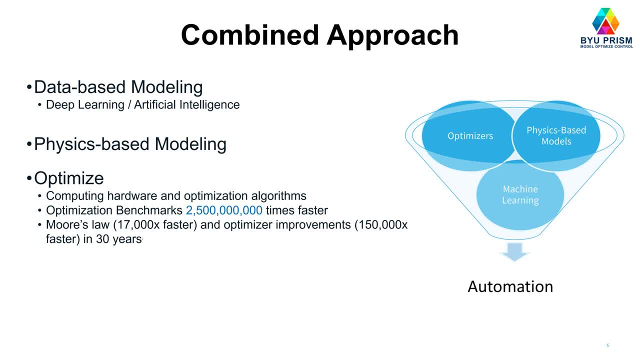 They've really progressed in the last 30 years. If we combine Moore's law, which has given us faster computing hardware, and then algorithm improvements, we can solve some of the same benchmark problems 2.5 billion times faster than we were able to 30 years ago. 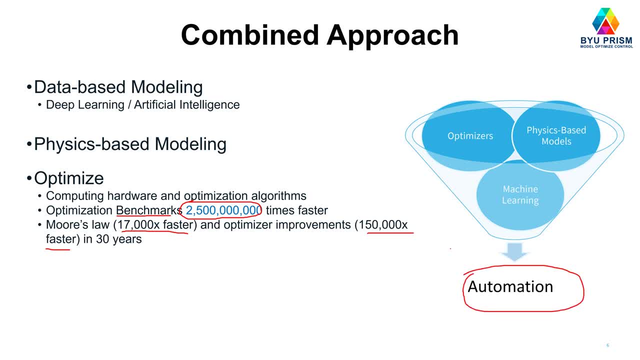 And so this has really opened the door for additional automation solutions, And in this course we're going to be combining machine learning physics-based models, also with optimization, And we're going to be looking at some of the best solutions from these models to be able 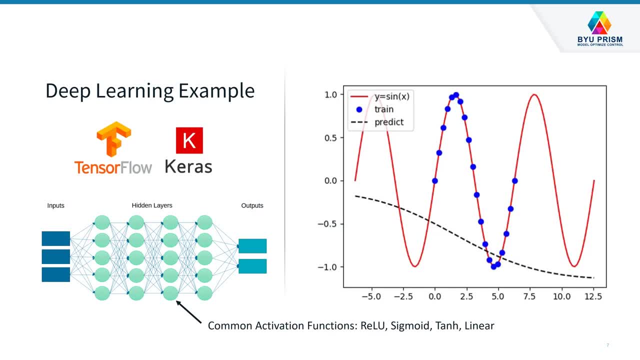 to come up with the best solution from these models. Now, if we look at some of the traditional ways to do machine learning, you might use a package like TensorFlow or Keras or PyTorch, And they're going to be common activation functions like rectified linear units, sigmoid. 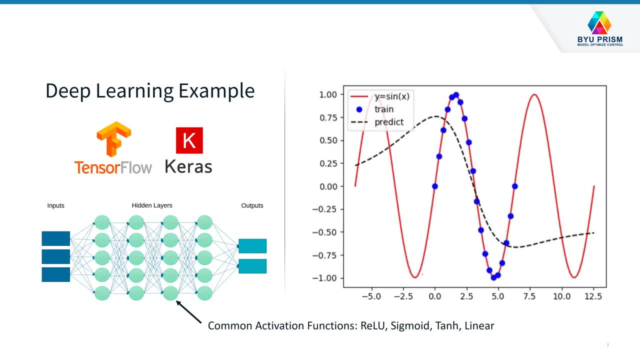 hyperbolic, tangent or linear, And so if we look at how we fit, you can see that over the data it's going to fit well, But the original function was sine of x, So we don't do that well at extrapolation outside of the training area. 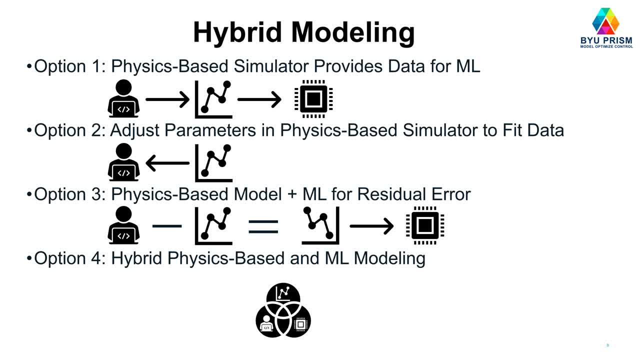 So we're going to be taking a hybrid approach to doing modeling and control, where, in the first option, we might use a physics-based simulator. In this case, let's say we have a person here that represents our physics-based a priori knowledge. 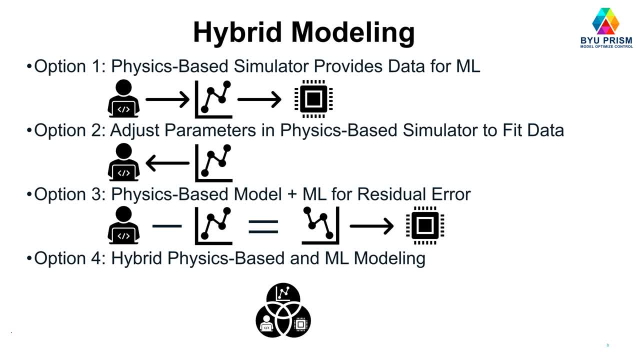 And then that person develops a model, Maybe generates some simulated data, and then feeds that to this processor icon, which is representative of machine learning, And so the machine learning learns the physics-based principles just through the output or the generated data. We can also use data to feed back into the physics-based simulator to adjust parameters. 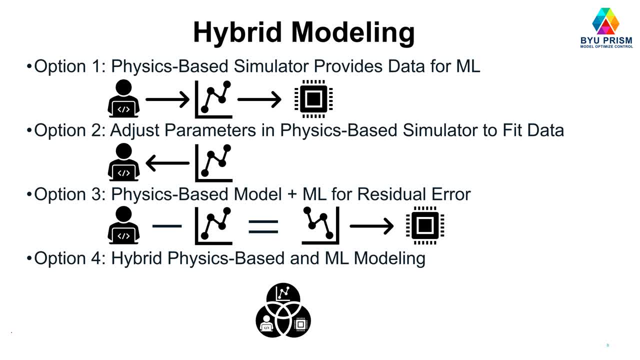 of that physics-based simulator. The next thing- Option three- is use a physics-based model and then look at the difference between the outputs, And that's called a residual, And then fit the remaining part that a physics-based model isn't able to cover with machine learning. 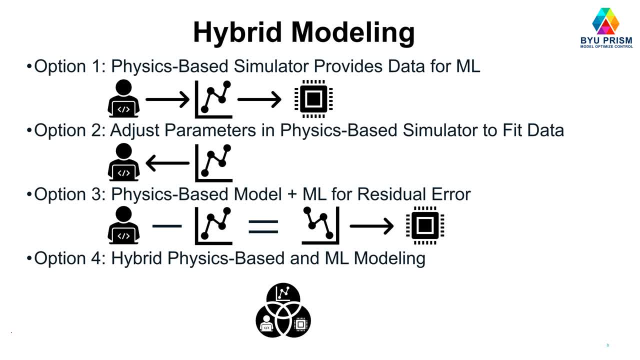 And so you have another layer of hybridization, or these hybrid models that you can create between physics-based and machine-learned models, Or, in a fourth option, when you're doing the fitting, you include physics-based and machine learning elements, And at the top of the second option, you include your additional element, which is the. 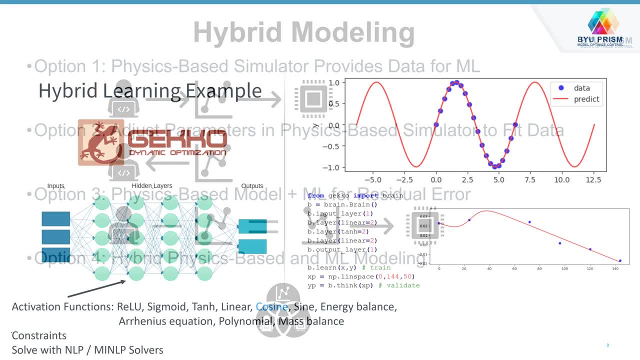 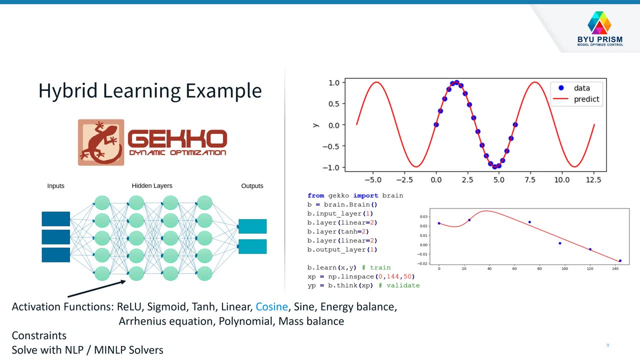 plus, And then you also include the radical elements. And then the third option is: you include the standard component, the element randomized components And another example- this is the sixth option- We're going to use our physics-based model And we're going to include the first and the only optical element. 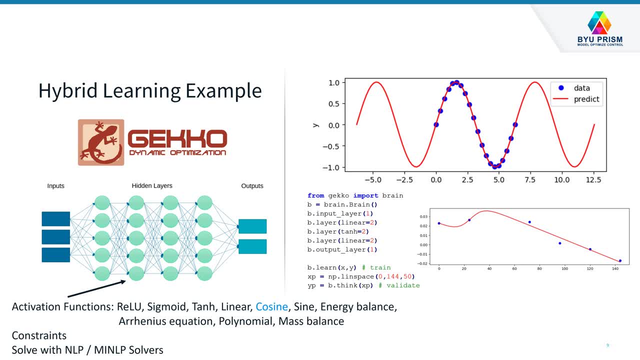 And then now let's do this in the second option, And that's just an example. see that by embedding a priori or fundamental knowledge into the system, like maybe you have a daily cycle and you can get better extrapolation and better model performance. 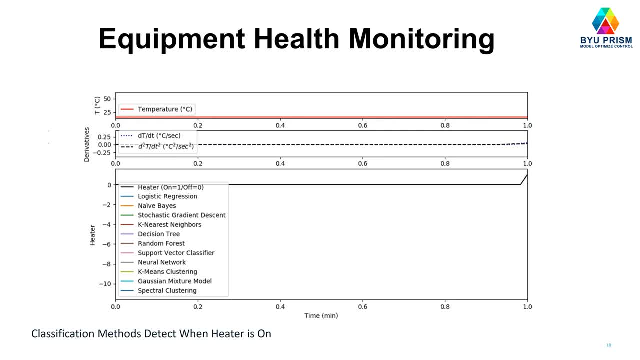 So here's an example of equipment health monitoring as well. This approach applies not only to control, but also to monitor and monitor equipment, which is a really important thing. with all of the equipment that goes into automation solutions, You want to make sure that. 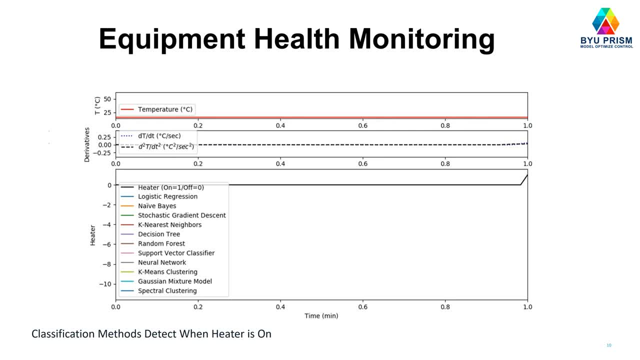 it's reliable And I'm going to show you just a result here, where the temperature is measured and the heater is on or off. in the bottom subplot We're going to generate some features which are the derivatives of temperature and use that with supervised learning methods. You. 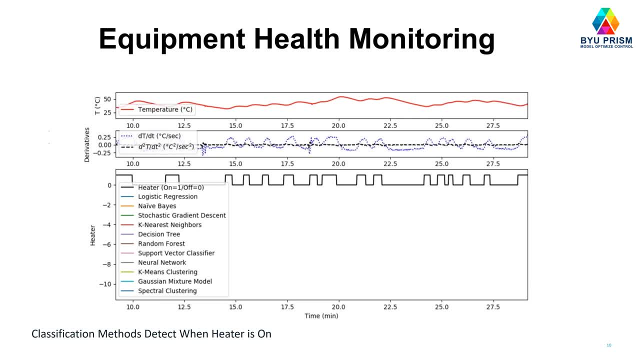 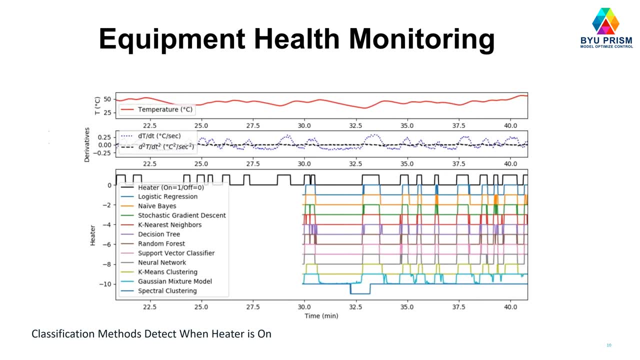 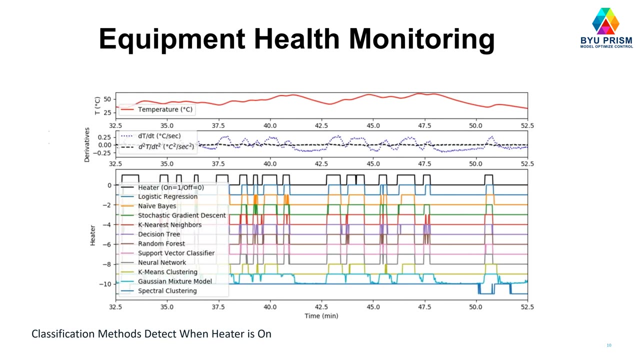 have eight of them here, and then three unsupervised learning methods to try to predict when the heater is on or off. So this is one of the example applications that we'll be doing in the course, using classification but also other machine learning approaches to develop these models. 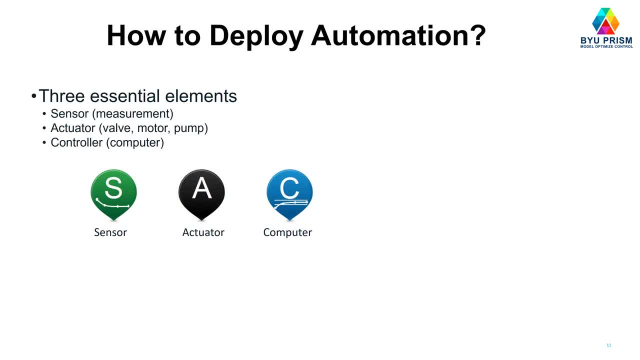 to accomplish the objectives. All right. so automation, even beyond monitoring, you have automation where you actually want to make a change to the process, And there are three essential elements for any automation solution. You've got to have the sensors, or else a digital twin of the process that takes the place of a sensor. You also need 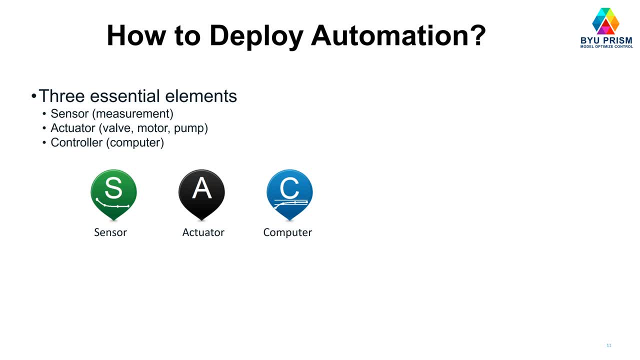 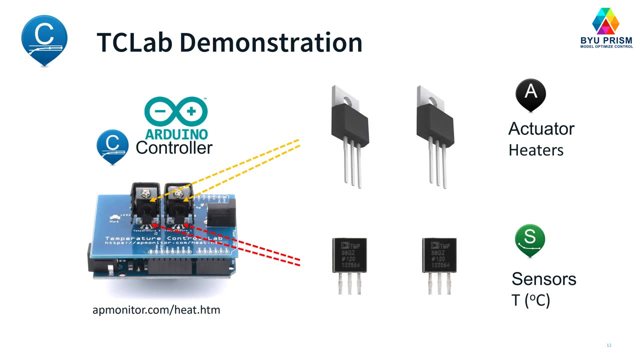 an actuator, something that will actually make a change to the process, like a valve, a motor, a pump. And then you need the algorithm, the controller, the computer that's able to take the sensor information and be able to recommend the best actuator movements. So with that, 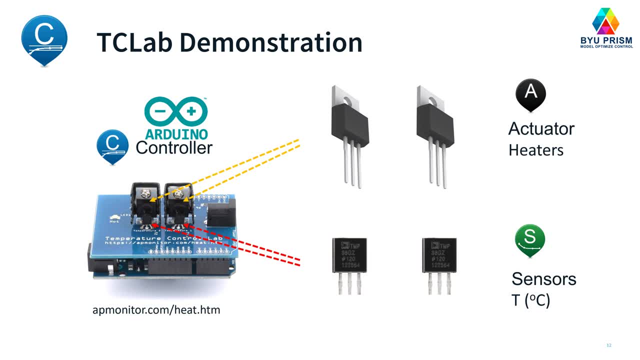 we'll have this Temperature Control Lab device that's available at the URL that you see below, where you have two heaters and two temperature sensors. So this is a multivariate control problem and we're going to be able to adjust the heaters to try to maintain. 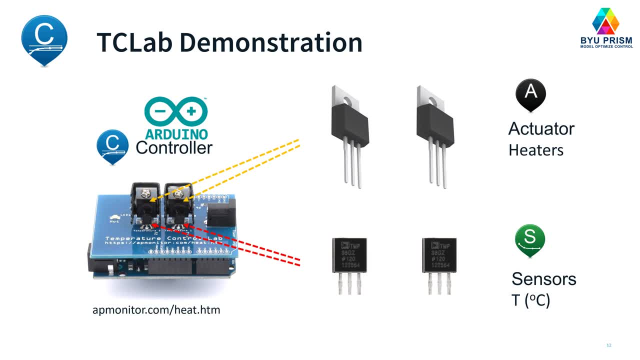 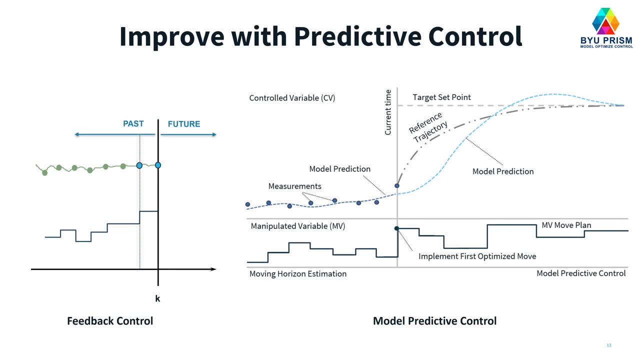 a desired temperature, much like a thermostat in a building. These are just two individual units that are next to each other and they affect each other as well, So there's some interesting interplay between the two. Now you may have had some background knowledge in feedback control, like proportional integral. 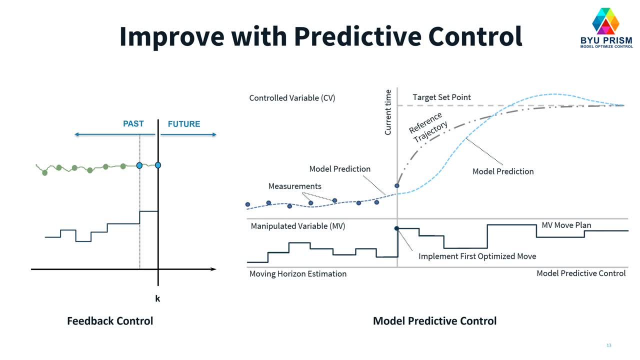 derivative controls and we'll compare that to this new approach, which is model predictive control, where we take the measurements and we align those with state estimation to the model And then, at the current time, we project forward into the future. There's a reference trajectory that we're trying to meet. 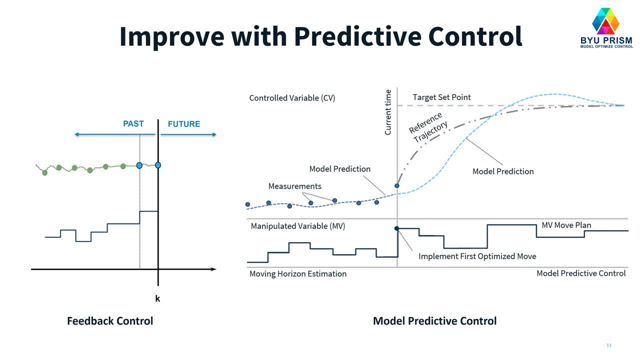 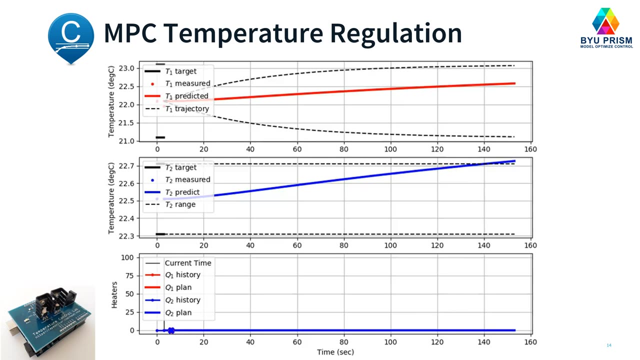 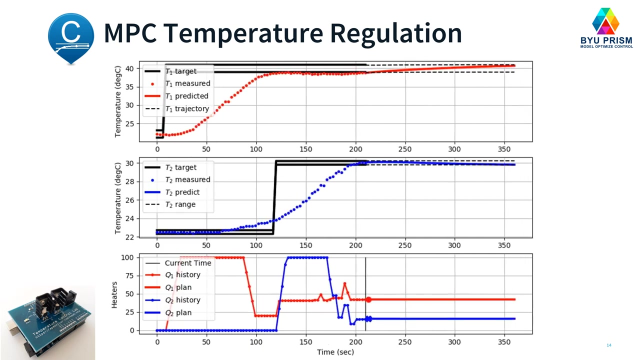 and you have your model prediction. You adjust the move plan with an optimizer until the model prediction gets as close as possible to the reference trajectory or maximizes profitability or minimizes costs. So this is an example with that Temperature Control Lab device looking forward into the future with the prediction horizon. 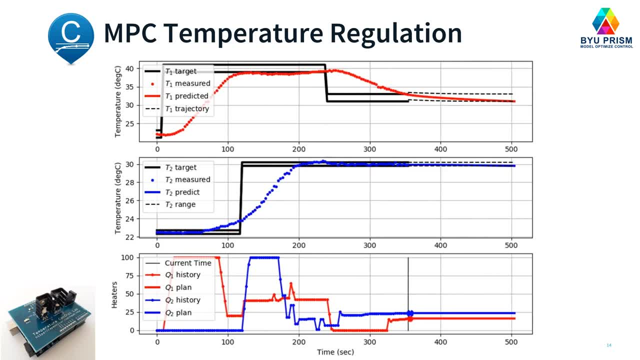 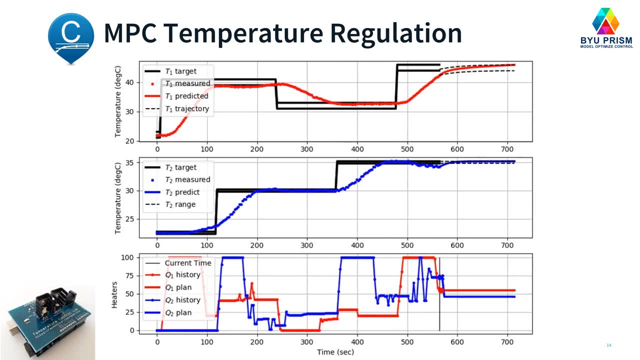 And then also on the very bottom you can see the move plan where you can see what the heaters are planning to do and you should be able to measure that in the future in maybe about 10,. let's see about two minutes in advance. 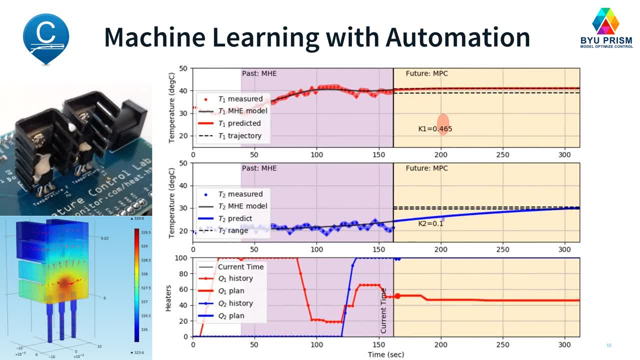 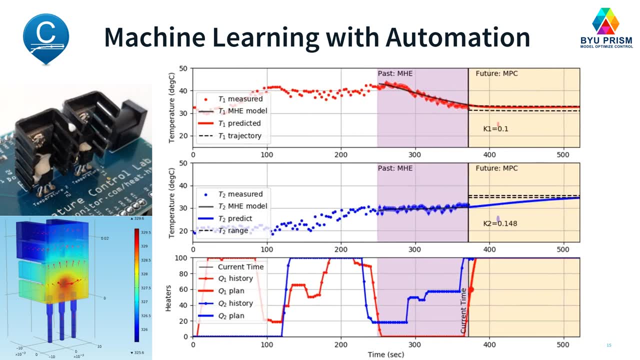 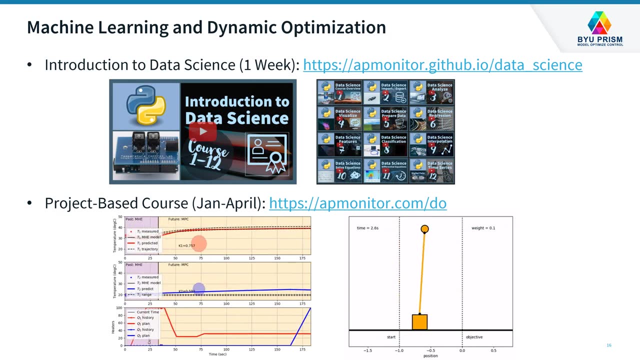 We're also going to combine that with moving horizon estimation or common filters to do an estimation of the current model state and parameters in the model. We'll then use that to then improve our model predictive control. So just getting started, I'd recommend go to the link there at the top of the page. 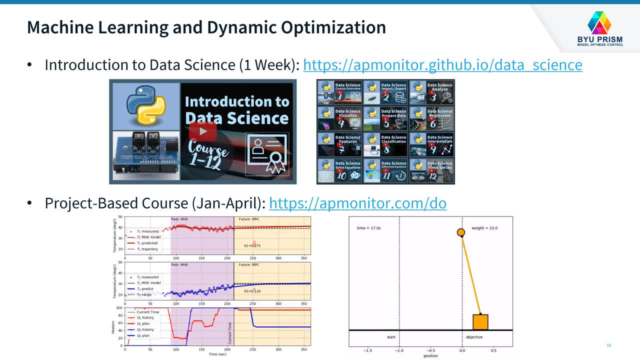 I've got a few extra slides there. These are quite useful. so, with the data science course, that'll help you review some of the Python packages and also help you get started with material. then we'll have the project-based course that goes January through April and there's the link there. 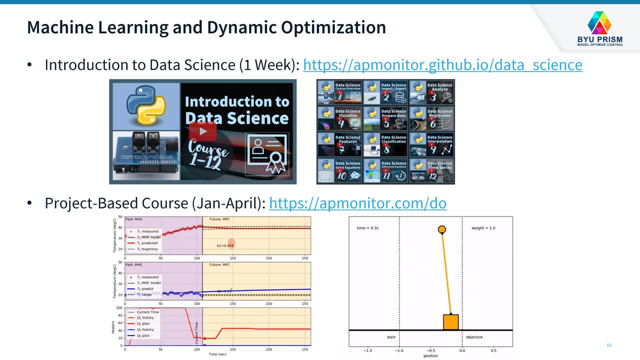 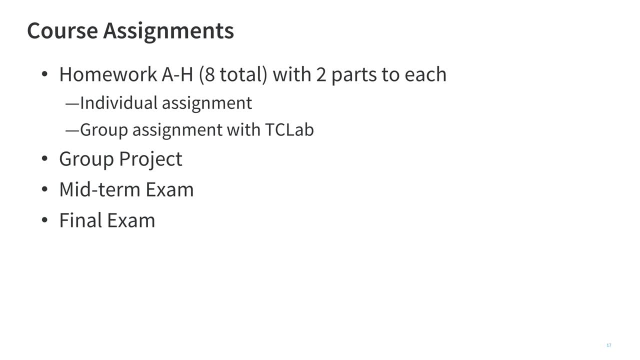 that you can visit in and get all of the course content. there are course assignments. these are going to be homework's, a through H, and there are two parts to each. the first part is an individual assignment that's more of like a simulation lab. the second one is going to be hands-on with the temperature. 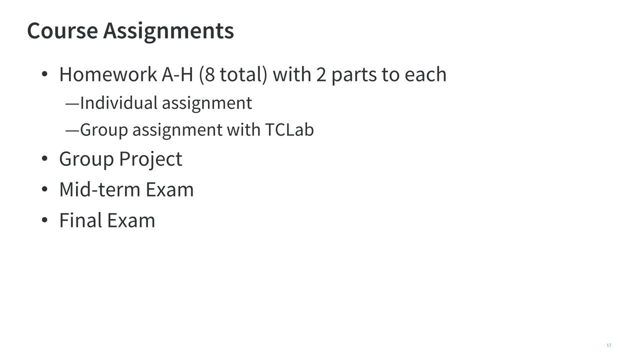 control lab, and you're welcome to work individually or in small groups. next, we're going to have a group project as well. so after we finish all of those exercises- and this is a self-selected group project where you can work with others who have similar interests to yours- also have a midterm and a final. 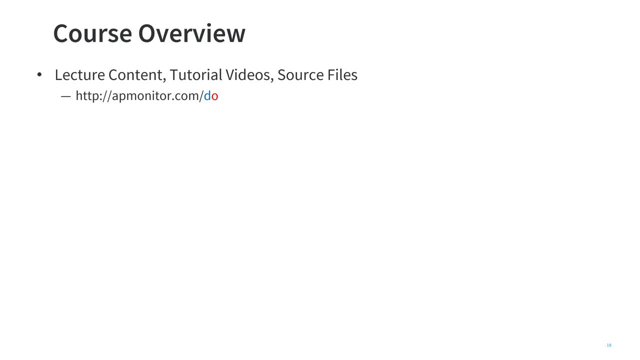 exam along the way. so there's the web address. this is the. includes the lecture content, tutorial videos, source files. also, if you get stuck, there are solution videos and solution files for all of the homeworks. main topics are dynamic modeling and digital twins, dynamic data machine learning and moving horizon estimation. 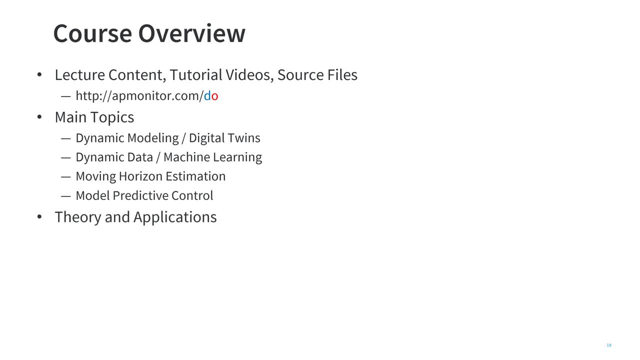 model, predictive control. we're going to be covering this with theory and applications. this is an engineering course. we're going to be heavily focused on how to apply these principles and extract value from the data. they're going to be numerical methods, will use a standard form, that for dynamic optimization, and they've also used 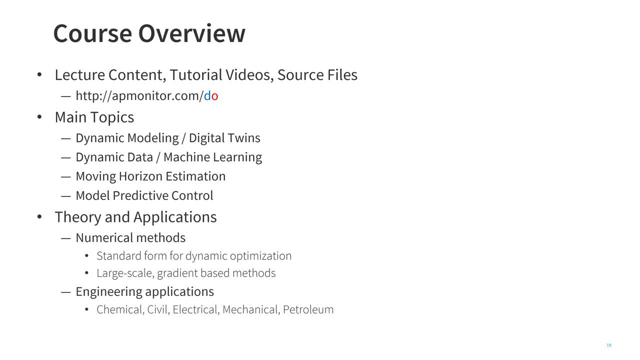 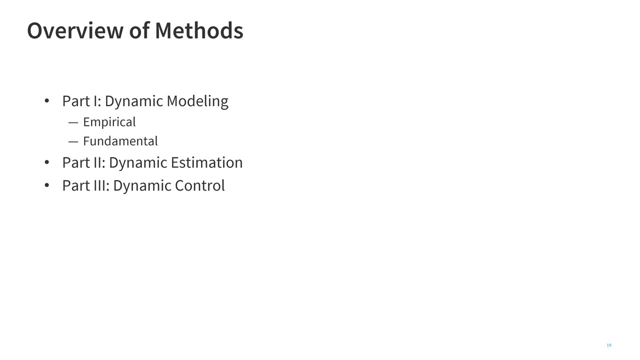 large-scale gradient-based solvers and many applications and chemical, civil, electrical, mechanical, petroleum, cyber security and others. ok, so let me go through the three parts of the course and a little bit more detail. we have part one, which is going to be dynamic modeling, and that includes 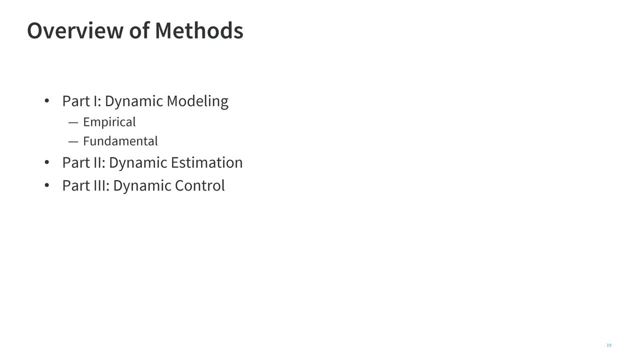 empirical or physics based models. we also have dynamic estimation and dynamic control. we're going to fit all of those into a standard framework where we have an objective function J, subject to equality constraints F, and inequality constraints G, and you can see the variables might be differential variables, such as X, or algebraic variables, such as Y, or parameters. 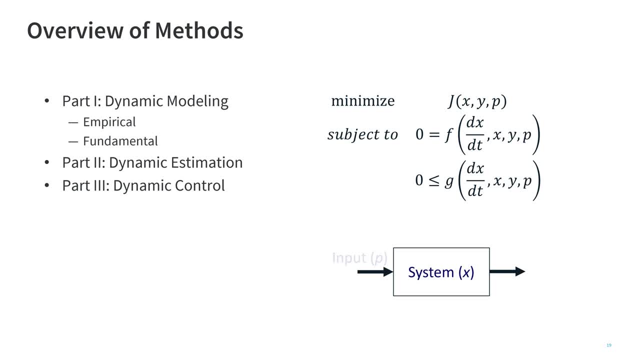 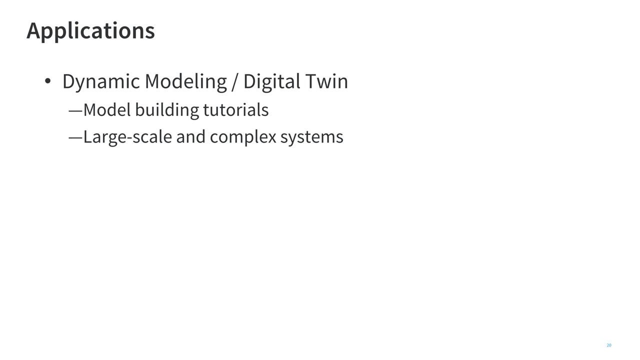 or inputs such as P. so the system is going to have inputs P, the- either we can adjust or we can measure, and then we're going to have predicted outputs Y and our system model might be a machine learn model or physics based model applications. we have dynamic modeling with digital twin. we're going to be 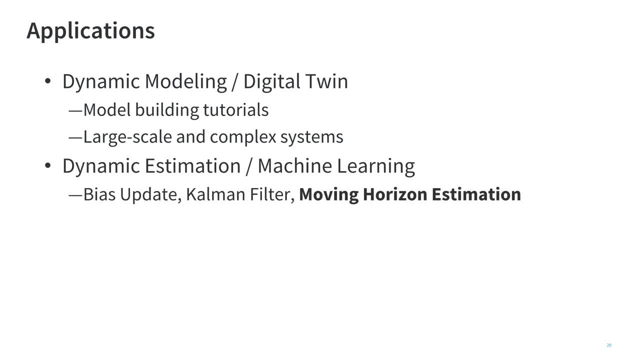 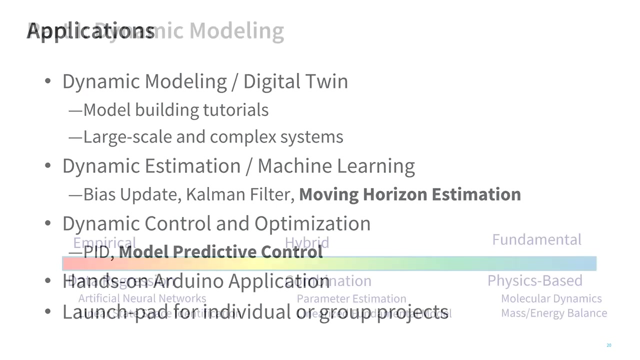 doing some model building tutorials with large-scale and complex systems and the next phase is this dynamic estimation: estimation with moving horizon estimation and then control and optimization with model predictive control and with this hands-on Arduino application for all of these, and really this is a launch pad for your individual or group projects. so just focusing a. 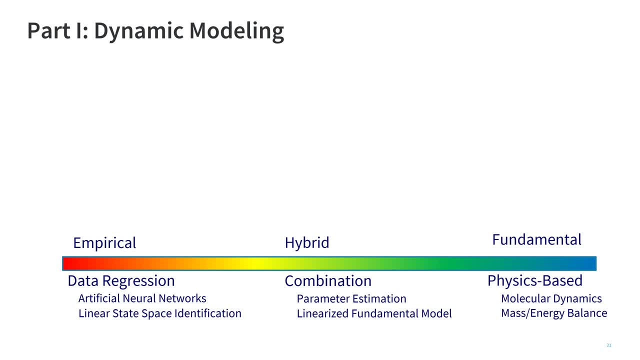 little bit more on the dynamic modeling. we're going to have a range between empirical and fundamental, using regression, physics based methods, or combination, which is the hybrid approach I mentioned. so you have the input and output and we're going to be minimizing subject to these constraints. now, in this case, we don't really have an objective function with simulation. we 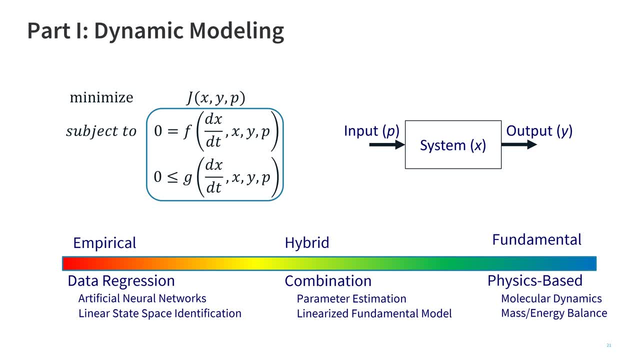 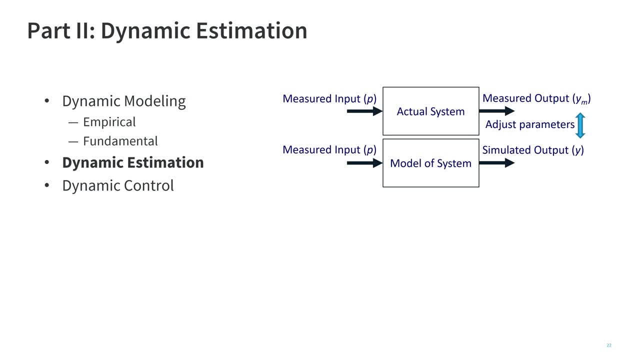 just have those equations that we're going to be solving to determine the values of X and Y. then we, when we go on to dynamic estimation estimation, we're going to have our digital twin and then we're going to have our dynamic estimation, which is below, and the actual system, which is above, and we have measured. 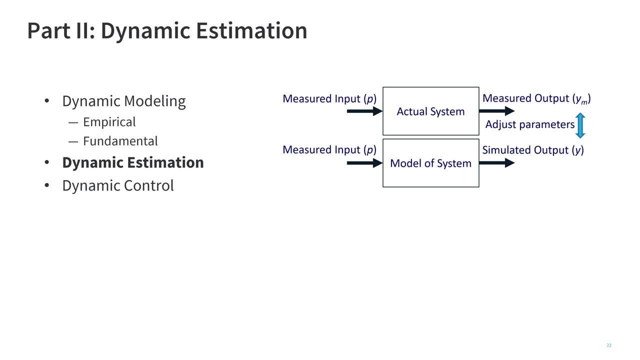 inputs P, and we're going to compare the measured output Y, sub M, to the simulated output Y and we're going to adjust parameters to make our model align with the measured output. now it's a slightly different form here, but really it's just the objective function. we're going to minimize some difference between the 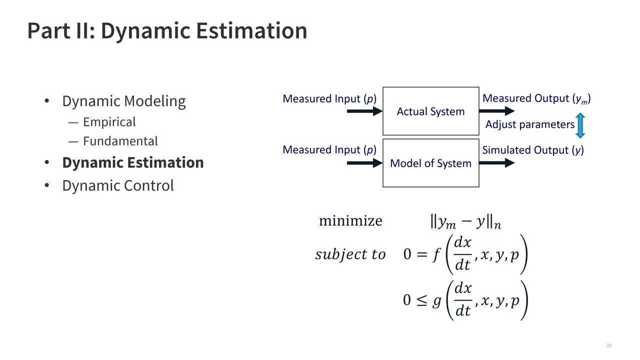 measured and predicted values and then we're going to have our dynamic estimation- which is below, and the actual system, which is below and the actual system. we're going to have our dynamic estimation check that out and we're going to have our model align with the predicted values by adjusting the parameters P or other types of unmeasured 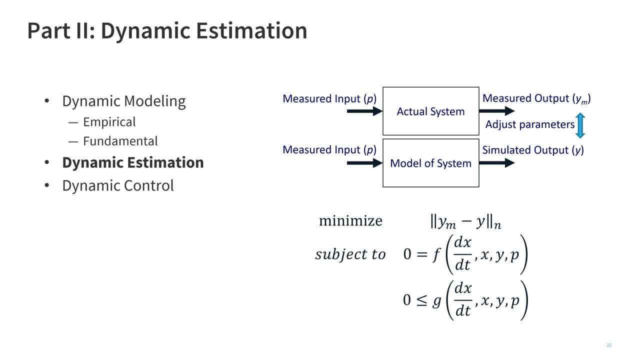 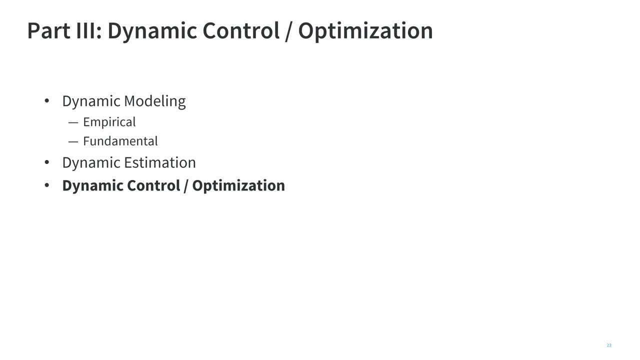 disturbances or other things that we can adjust with the model. we may even determine what model to use. from machine learning then going on to dynamic control and optimization, we're going to change the form a little bit. so now, instead of trying to synchronize to measurements, we're trying to align to some reference trajectory or 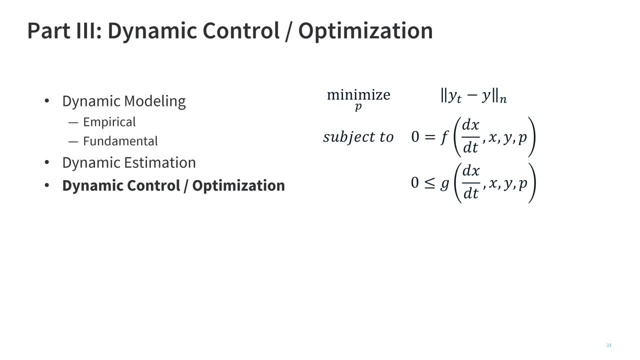 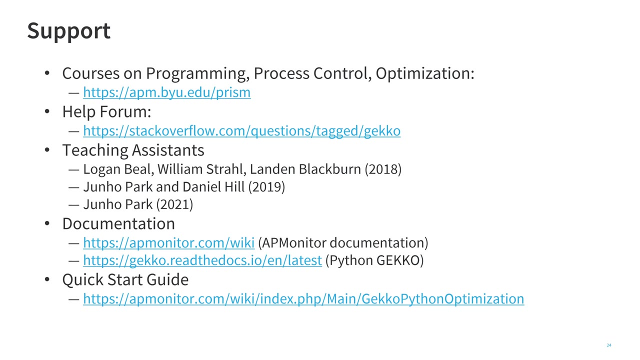 economic statement of profitability or minimize cost. again, we're going to use the same system, models and so, along the way, this is a lot of material and you might be coming at this course with a different background. there are many helps that are available if you need to start with programming, for example, and 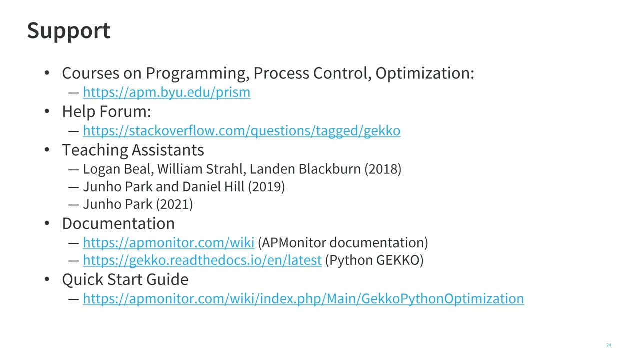 get some help with Python. there's a course available for that as well, to start from almost zero experience. there's also a help forum online on Stack Overflow. just search for any of the questions that are tagged gecko. there are also teaching assistants that are going to be able to help. I really 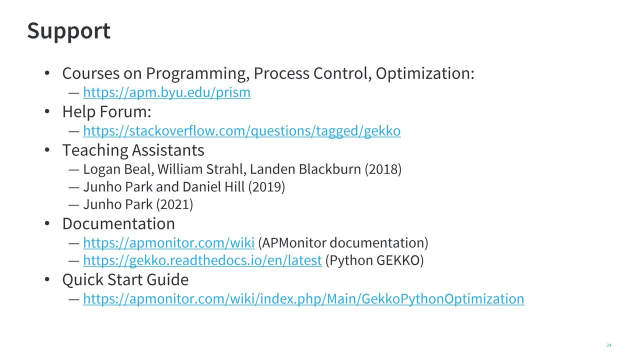 appreciate those that have helped in the past and we've got Junho helping this year documentation. you're going to be able to help. I really appreciate those that have helped in the past and we've got Junho helping this year documentation documentation. there's a website for documentation, for if you monitor a gecko, we're gonna be. 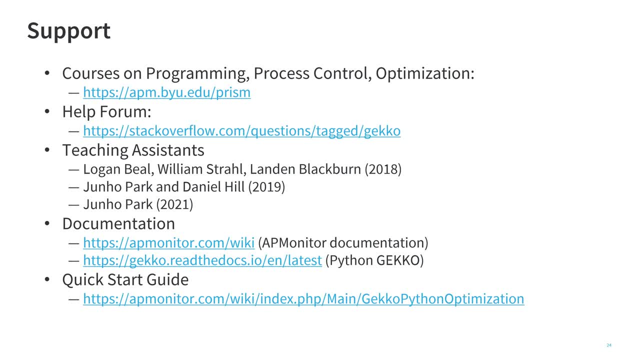 there's a website for documentation for if you monitor a gecko, we're gonna be using those packages, but there are also other packages like scikit-learn Keras using those packages. but there are also other packages like scikit-learn Keras tensorflow and pie torch that we're going to be using and they're excellent. 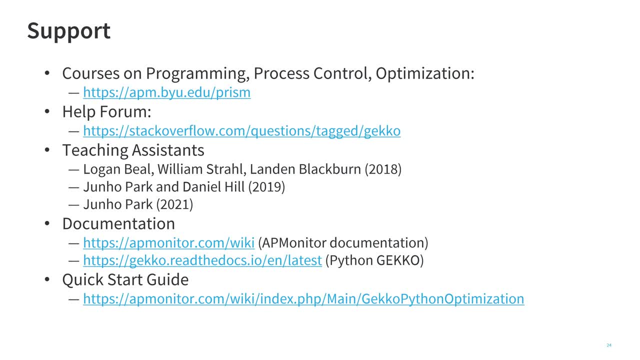 tensorflow and pie torch that we're going to be using and they're excellent documentation resources online also there's a quick start guide. if you just documentation resources online also, there's a quick start guide. if you just want kind of the brief version of this course, I'd recommend that quick start. 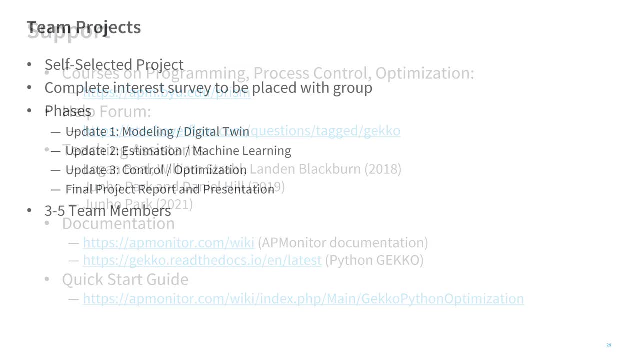 want kind of the brief version of this course. I'd recommend that quick start guide with 18 example problems. okay, a little bit more about team projects guide with 18 example problems. okay, a little bit more about team projects guide with 18 example problems. okay, a little bit more about team projects. these are going to be self-selected projects. 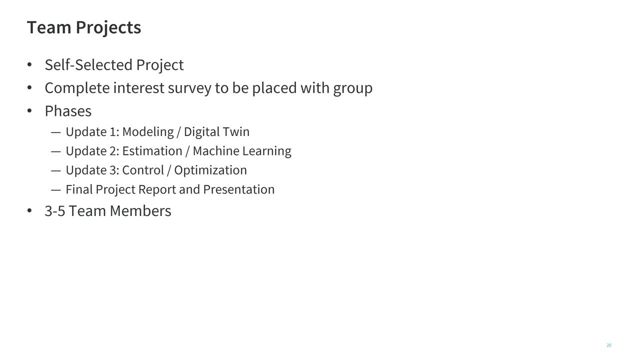 these are going to be self-selected projects. these are going to be self-selected projects midway through the course. we're midway through the course. we're midway through the course. we're gonna have you complete an interest survey to gonna have you complete an interest survey to gonna have you complete an interest survey to be placed with a group, with those. 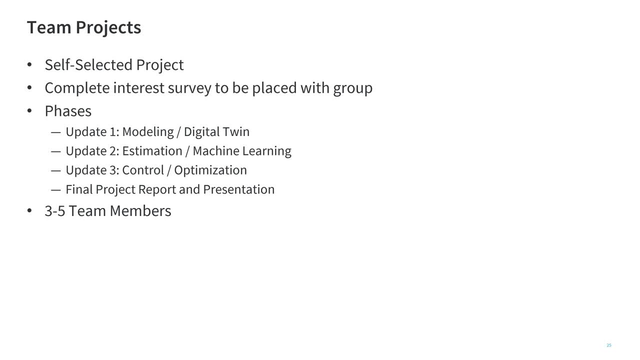 be placed with a group with those. be placed with a group with those from industry or academia with similar from industry or academia, with similar from industry or academia, with similar interest to yours. we're gonna go interest to yours, we're gonna go interest to yours. we're gonna go through this course in a number of 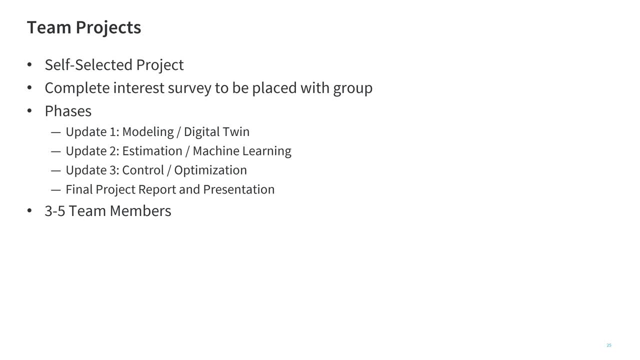 through this course, in a number of through this course, in a number of different updates or phases. we have the different updates or phases. we have the different updates or phases we have. the first phase is to develop some first phase is to develop some first phase is to develop some mathematical representation of your system. 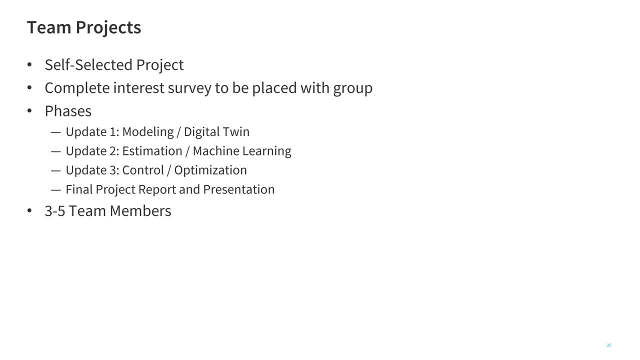 mathematical representation of your system. mathematical representation of your system. now this could be a physical piece. now, this could be a physical piece. now, this could be a physical piece of hardware that you're trying to control, of hardware that you're trying to control, of hardware that you're trying to control, like, maybe, a self balancing robot. 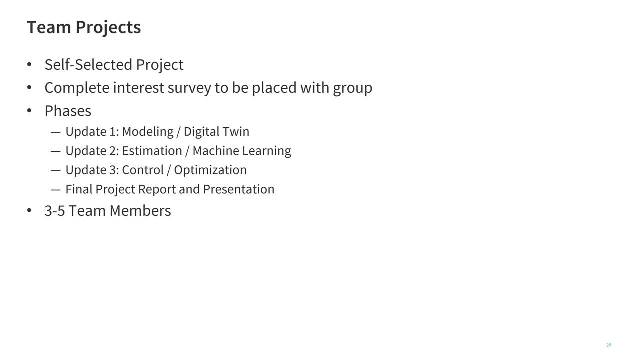 like, maybe a self balancing robot. like, maybe a self balancing robot or other type of device, the very first or other type of device, the very first or other type of device. the very first thing we want to do is create a. thing we want to do is create a. 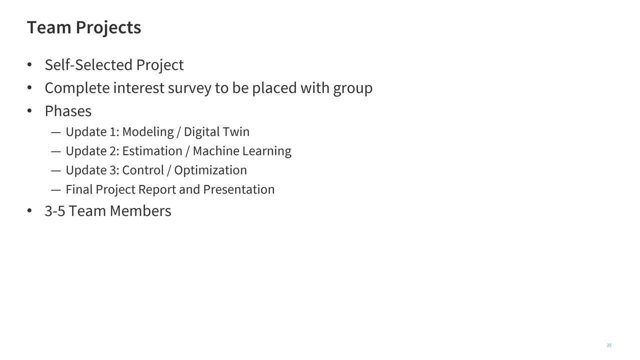 thing we want to do is create a mathematical representation of what you're mathematical representation of what you're mathematical representation of what you're trying to control or optimize- a trying to control or optimize, a trying to control or optimize. a second update is going to be using data. 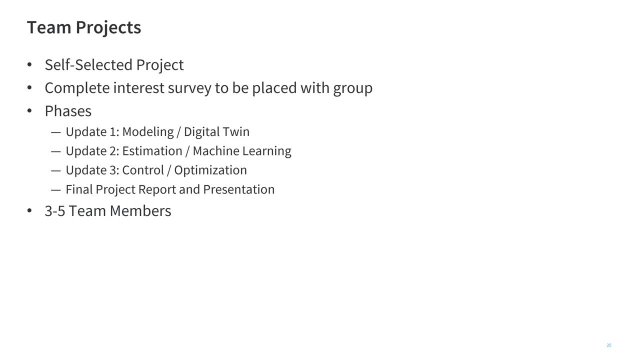 second update is going to be using data. second update is going to be using data from that device or data that you have from that device, or data that you have from that device or data that you have available from your process to be able, available from your process to be able. 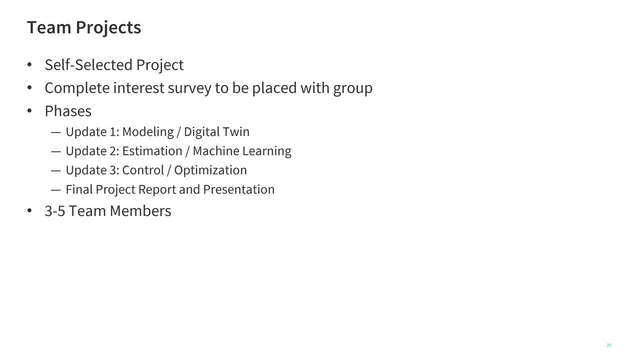 available from your process to be able to improve the model or perform machine. to improve the model or perform machine. to improve the model or perform machine learning. classification or regression learning. classification or regression learning. classification or regression methods. update 3 is going to be control methods. update 3 is going to be control. 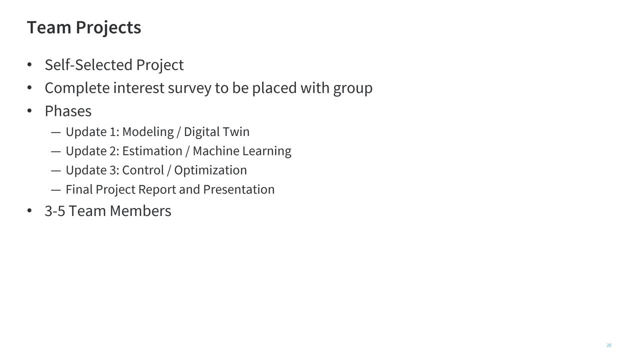 methods. update 3 is going to be control and optimization- we're going to take and optimization- we're going to take and optimization- we're going to take those models and then have an advisory those models and then have an advisory those models and then have an advisory system or some type of automatic. 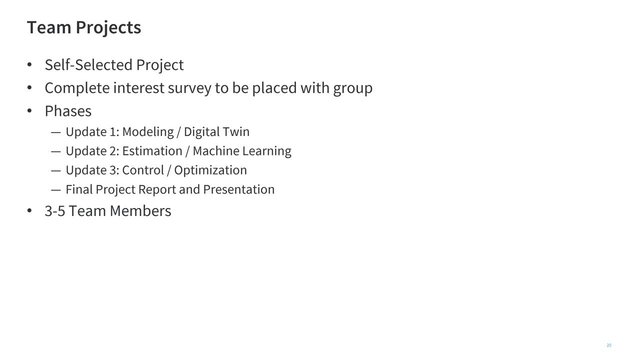 system or some type of automatic system or some type of automatic. the final project will include a report. the final project will include a report. the final project will include a report and presentation. you'll be able to share and presentation. you'll be able to share and presentation. you'll be able to share your results with others in the course. 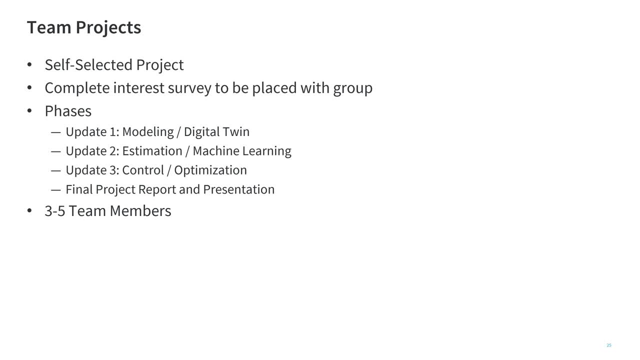 your results with others in the course. your results with others in the course. i recommend teams of three to five team. i recommend teams of three to five team. i recommend teams of three to five team members. members: members that include participants from industry. that include participants from industry. 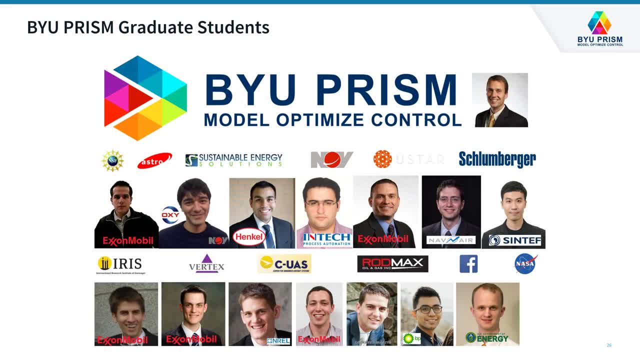 that include participants from industry and academia also. i'd like to just thank all the also. i'd like to just thank all the also. i'd like to just thank all the students that i've had in the prism students that i've had in the prism students that i've had in the prism research group. these are just the. 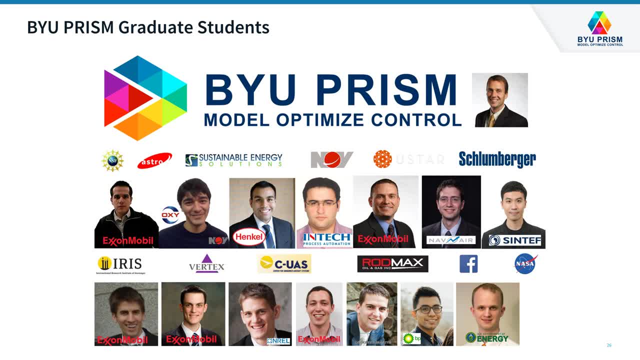 research group. these are just the research group, these are just the graduate students, but we've had many graduate students, but we've had many graduate students, but we've had many other undergraduate research assistants, other undergraduate research assistants, other undergraduate research assistants as well, as well, as well. the byu prism group. prism stands for. 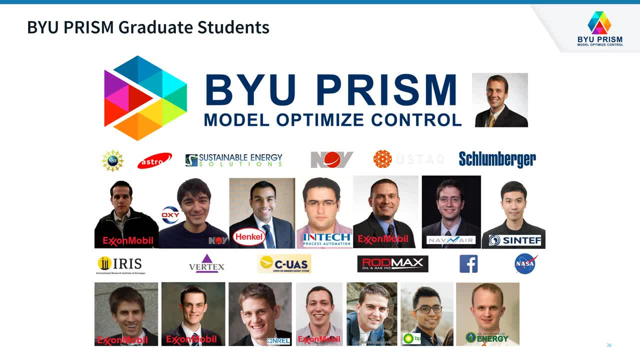 the byu prism group. prism stands for the byu prism group, prism stands for process research, intelligence systems, process research, intelligence systems, process research, intelligence systems modeling, modeling, modeling group and we've had a number of very group and we've had a number of very group and we've had a number of very fantastic graduate students have helped.